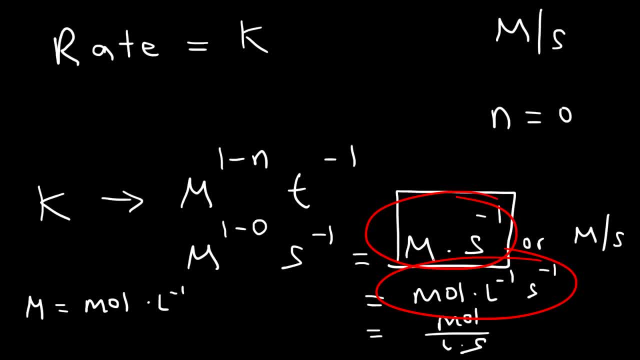 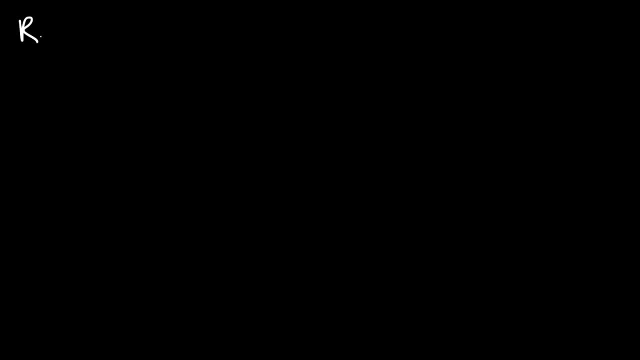 but I'm going to leave it like this and like this, Because on a typical test you might see it like that. Now let's work on another example. So let's say: if we have this particular rate, law expression rate is equal to k times A. 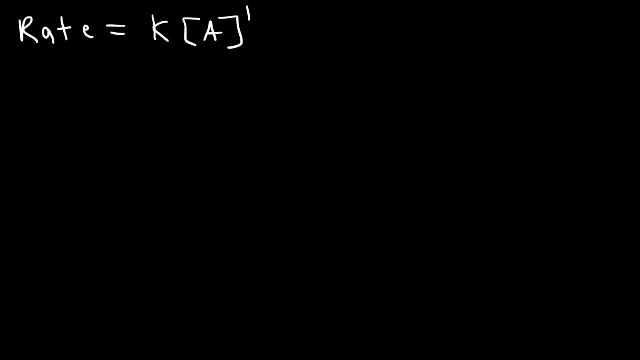 where that is the concentration of A and it's raised to the first power. So it's first order with respect to A and it's first order overall. And let's say you're given the units of the rate of the reaction and it's moles, times liters to the minus 1, times minutes to the minus 1.. 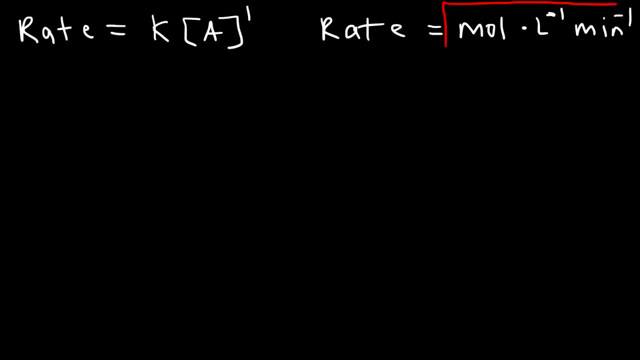 So notice how the unit of rate is written. So for k we want to write it in a similar fashion. So let's start with the formula. The units of k is going to be molarity raised to the 1 minus n times the time raised to the minus 1.. 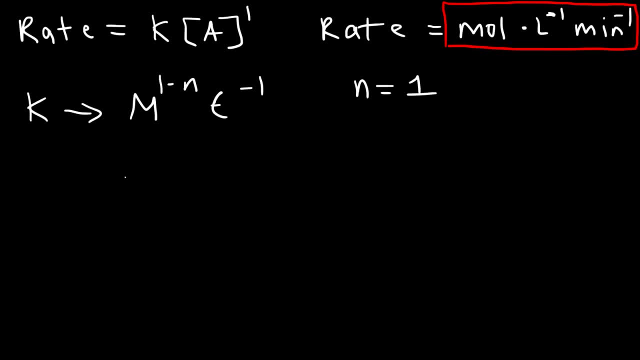 So it's first order overall, which means that n is equal to 1.. So it's going to be 1 minus 1, and the time is in minutes, So we can replace t with minutes. 1 minus 1 is 0, so it's m to the 0 times, minutes to the minus 1.. 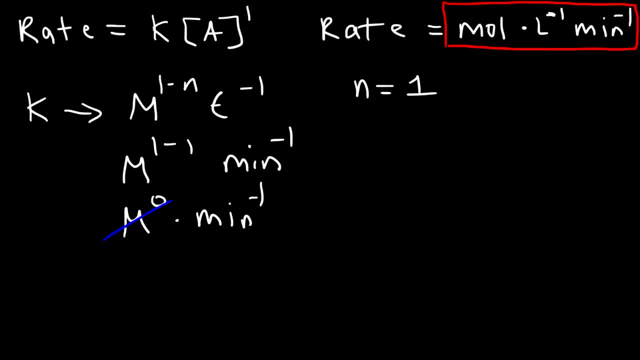 And so anything raised to the 0 power is 1, so we can get rid of this. So in this example the units of k is simply minutes to the negative 1 power or 1 over minutes. Now here's another example. 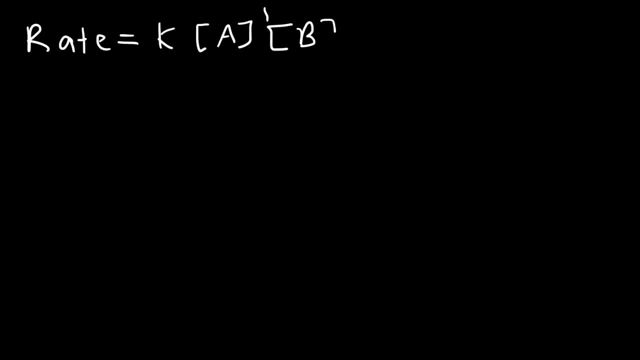 This time it's first order with respect to a and first order with respect to b. 1 plus 1 is 2, so it's second order overall. And let's say the rate expression is given to you in terms of the units: molarity per hour. 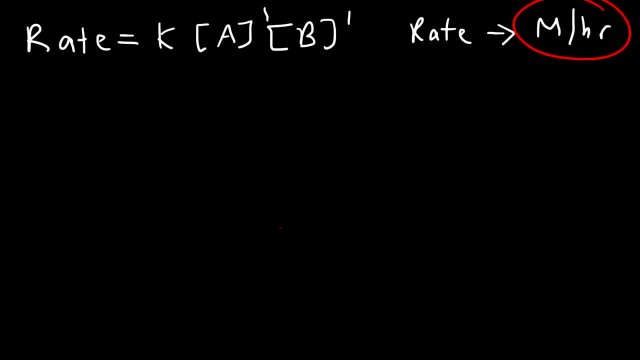 So I'm going to write the units of k in a similar way, using molarity instead of moles per liter. So let's start with the formula. So let's start with the formula. So let's start with the formula. So it's going to be m raised to the 1 minus n times t raised to the minus 1.. 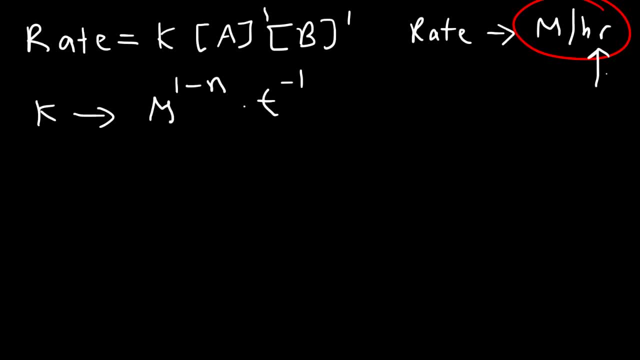 So this time the units of time is hours as opposed to seconds or minutes, And because it's second order, overall n is 2.. So it's going to be 1 minus 2, and then hours to the minus 1.. 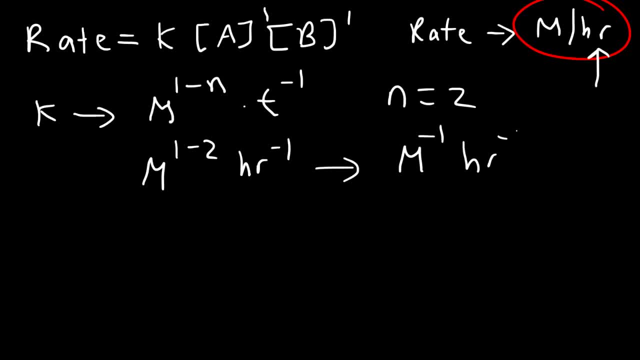 So 1 minus 2 is negative 1.. And so what we have now is We have molarity on the bottom, because it's to the minus 1, and hours is in the denominator as well. Now keep in mind that molarity is moles per liter. 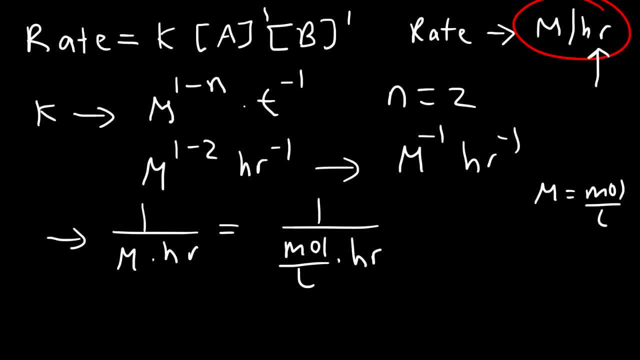 So we can replace capital M with moles per liter. Now I'm going to multiply the top and the bottom by liters, And so the unit is going to be liters on top divided by moles per liter. So that's how I'm going to write it. 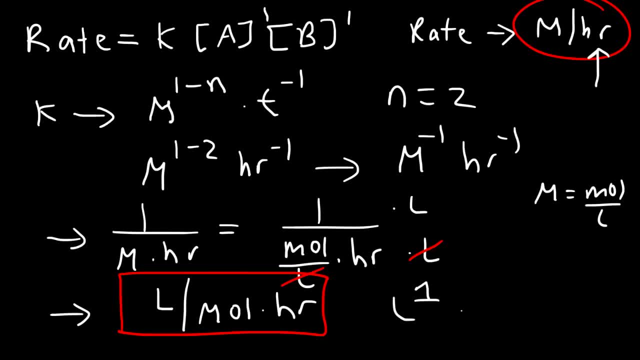 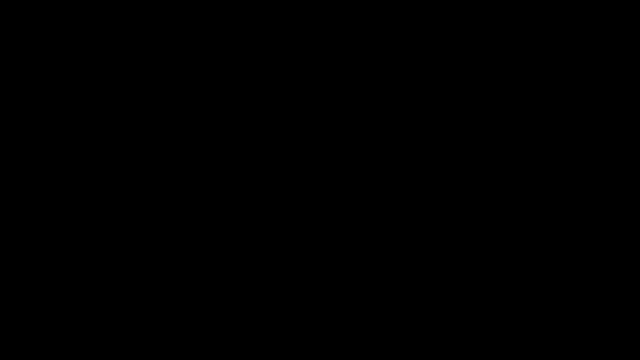 Now, if you write it like this: liters to the first power, times moles to the negative 1, times hours to the negative 1, it's still correct. You can write it that way if you want. Actually, before I get rid of this page, 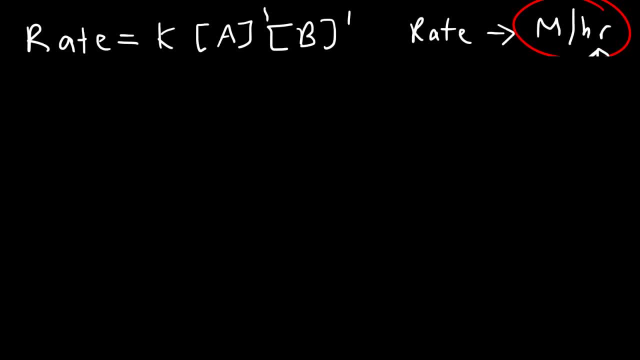 I want to show you how to get the answer without using the formula. So if you ever forget what the formula is, here's what you need to do. In the rate law expression, isolate K. So that means we need to divide both sides by AB. 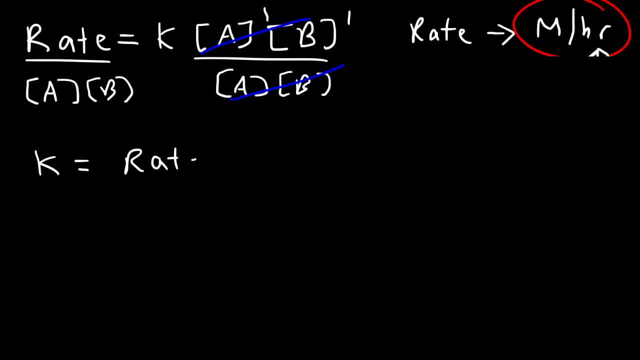 So K is equal to rate over A times B And then replace everything. So the rate is in molarity per hour And the concentration is always going to be in molarity. So the concentration of A is in molarity and B is in molarity. 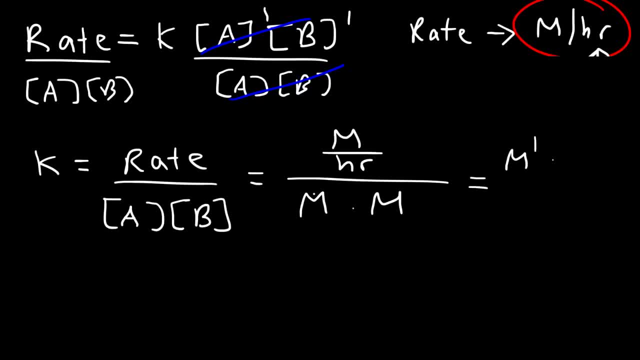 So molarity per hour. you can write that as M to the first power times, hours, to the negative 1.. And it might be easier to do it that way. So notice that we can cancel M. Now I'm going to take this M and move it to the top. 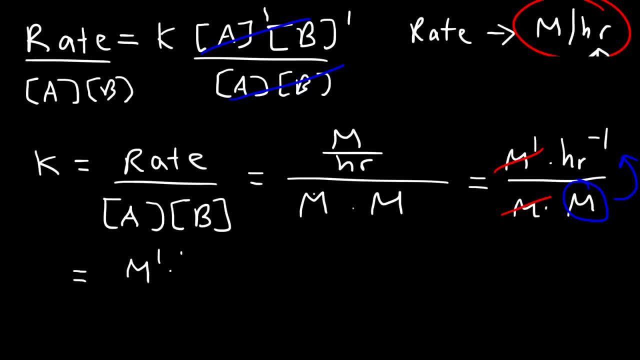 So it's going to be M to the first power times- actually not to the first power- to the negative 1 power. Whenever you move something from the bottom to the top, the exponent changes signs. So it's going to change from positive 1 to negative 1.. 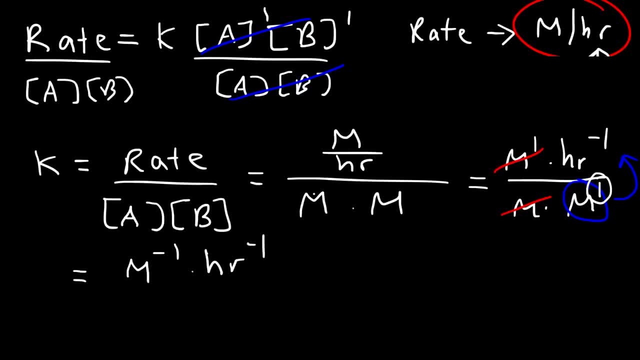 So it's M to the negative 1, hours to the negative 1.. So you can leave it like that. Now keep in mind that molarity is moles per liter. So M to the first power is technically moles to the first power. 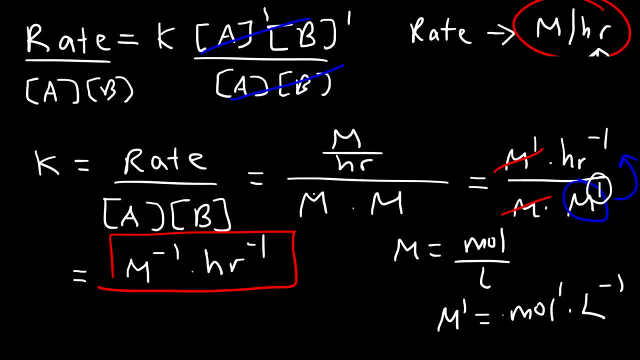 times liters to the negative 1.. So if we multiply all the exponents by negative 1, M to the negative 1 is going to be moles to the negative 1, times liters to the positive 1.. And we've got to use this one for this example. 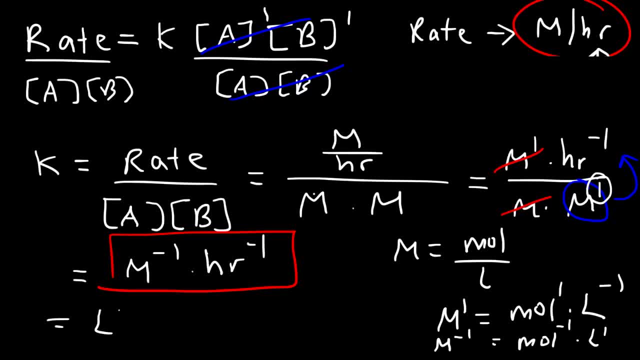 So I'm going to replace M to the negative 1 with liters to the first power, times moles to the negative 1 power, And then we have hours to the negative 1.. So this gives us the same unit that we had in the last example. 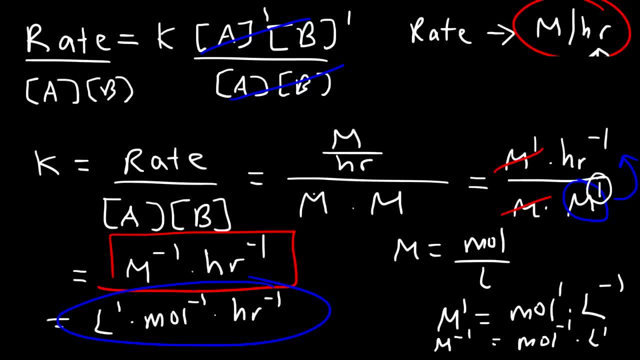 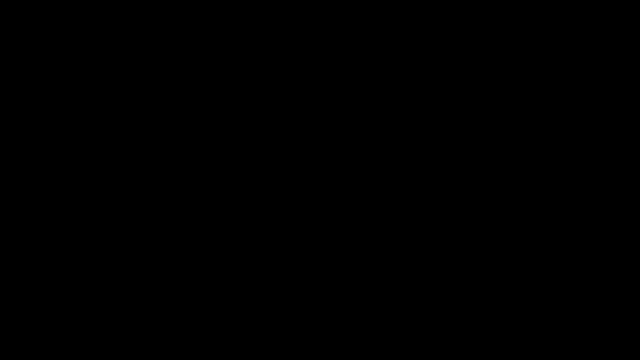 So the formula works And it's up to you to decide which method works better for you. Now let's work on another example. This time I want you to use the formula and I want you to confirm your answer by solving for K. 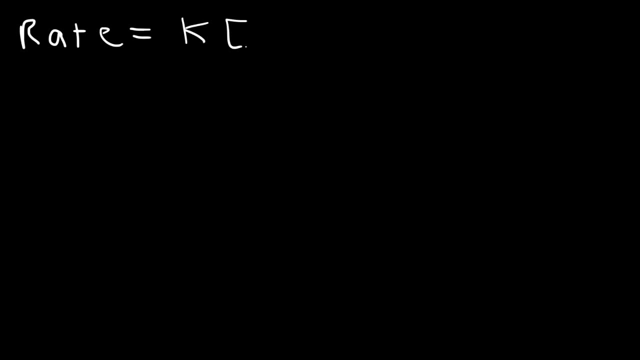 So rate is going to equal K times A to the first power, times B to the second power. So it's first order with respect to A, second order with respect to B. So it's first order with respect to A and it's third order overall. 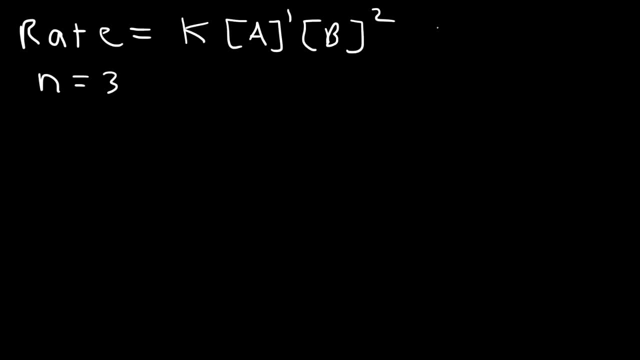 which means that N is equal to 3.. And let's say that the unit of rate or the rate of reaction, it's going to be moles to the first power, times, liters to the negative 1, times, let's say days, to the negative 1.. 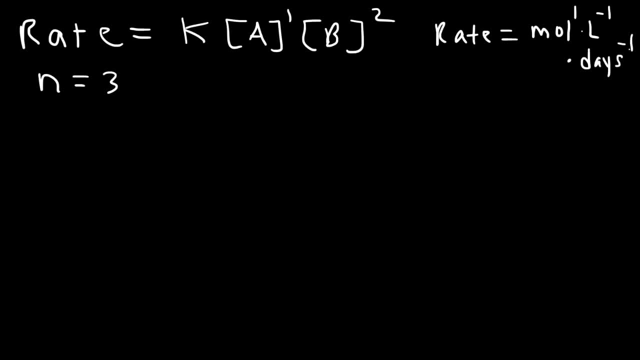 So it's a very slow reaction. So go ahead and use the formula to get the units of K. So it's going to be M raised to the 1 minus N times T to the minus 1.. So we can see that the time is in days. 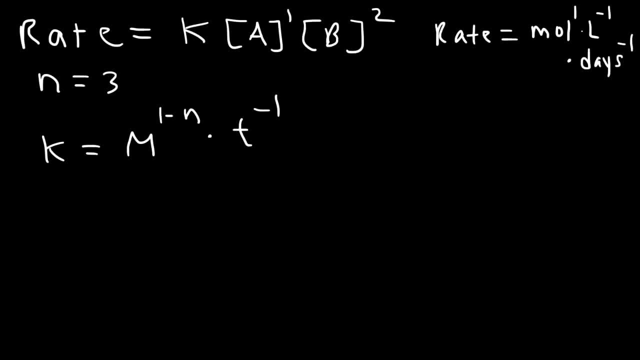 So we're going to replace T with days instead of seconds, minutes or hours, And N is 3.. So it's M raised to the 1 minus 3, and then days to the minus 1.. So 1 minus 3 is negative 2.. 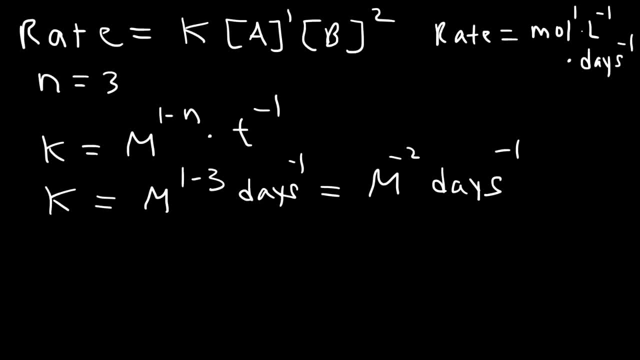 So, if you want to, you could leave the answer like this: If you have a multiple choice test, you have to adjust the answer in a way that matches your multiple choice answers. So you can leave it like this, or if you want to change it, that's cool. 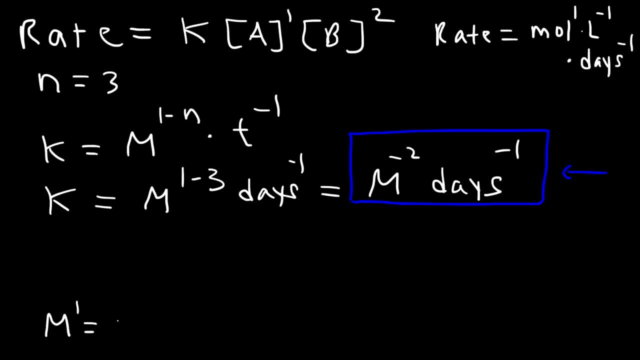 So keep in mind that molarity to the first power is moles to the first power times liters to the negative 1.. Now I have molarity to the negative 2, so I'm going to raise each exponent to the negative 2 power. 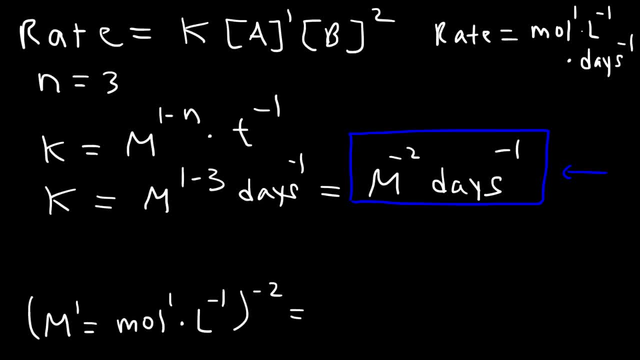 So I'm going to multiply. I multiply 1 by negative 2, and so this becomes M to the negative 2.. And then this is also 1 times negative 2, so this becomes moles to the minus 2.. And negative 1 times negative 2 is positive 2.. 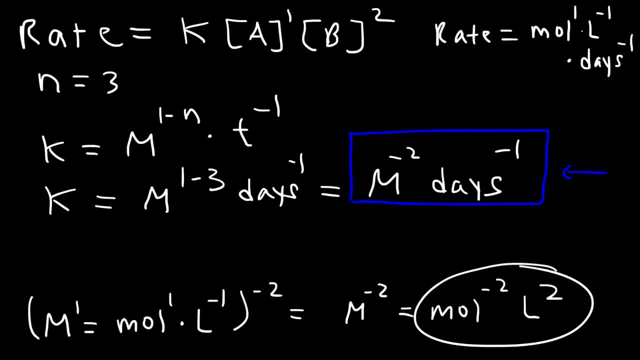 So moles to the negative 2, I can replace it with this, So I can write my answer as liters: squared times moles to the minus 2, times days to the minus 1.. So you can also write the answer like this, if you want. 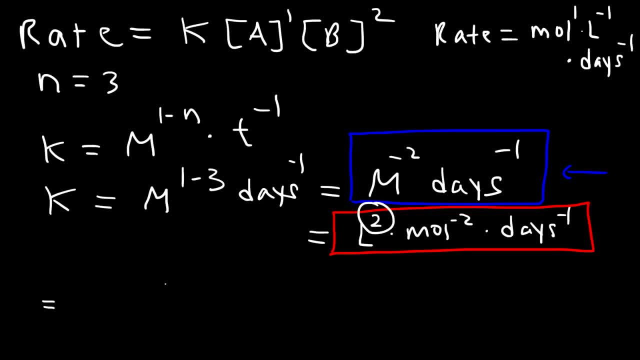 Now, if you want to write it as a fraction, everything with a positive exponent, put it on top, So we have liters squared. Everything with a negative exponent, move it to the bottom, And if you do that, the exponent is going to change from negative to positive. 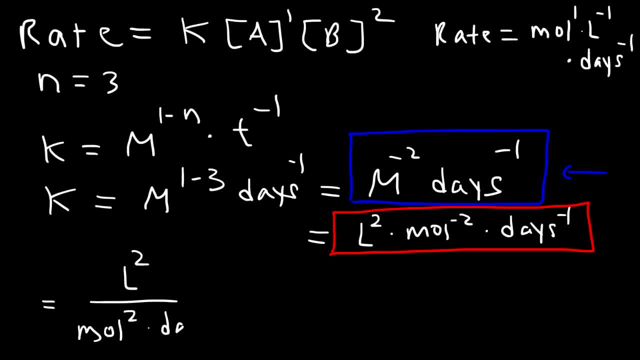 So it could be moles squared on the bottom times, days to the first power. So you can write this as it's liters squared per moles squared times, days Or times a day. So you can also write it like that. Now let's solve for K. 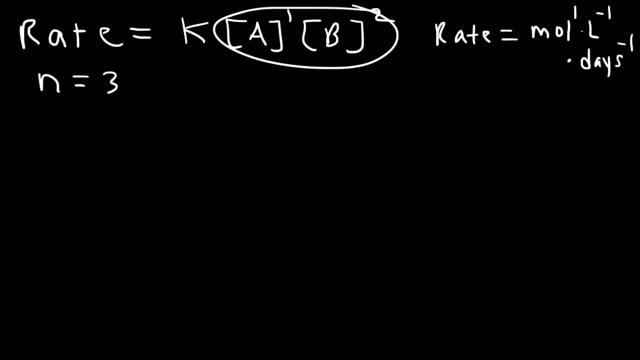 So to get K by itself, we need to divide both sides by this expression. So K is going to be the stuff on the left, which is the rate of the reaction, divided by the stuff on the left, and we're going to write: except K. 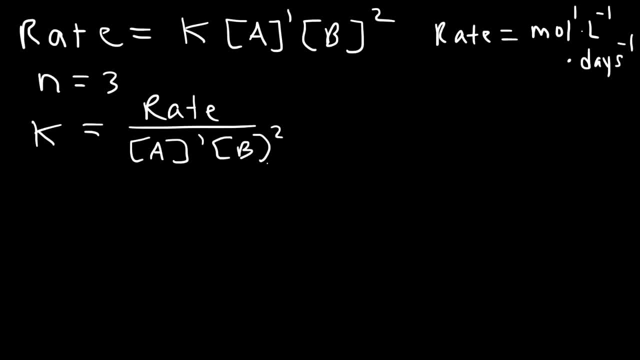 So that's A to the first power, B to the second power. So we already have the units of the rate. So it's moles times liters to the minus 1, which this part is molarity. So I'm just going to replace that with M for now.